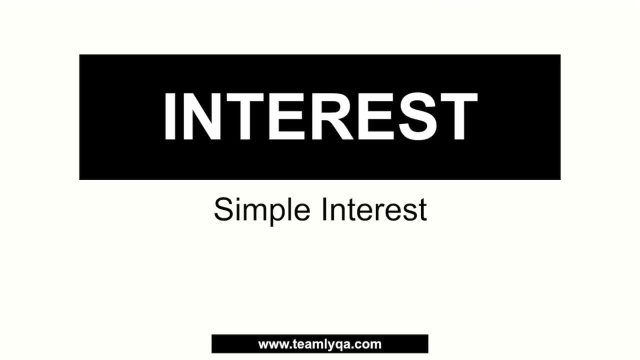 guys, I'll see you in a bit, So let's start with the lesson of simple interest. Again, if you haven't seen the older videos on this topic, just click here on the top on the i button so you can watch it. Let's start with the formula. 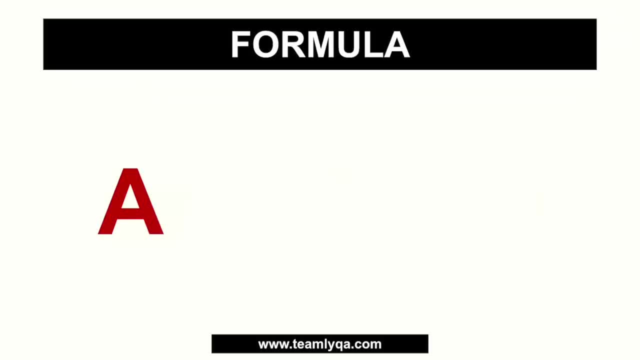 Now, if you go by the book, the real formula of simple interest would look like this: A is equal to P times the quantity 1 plus RT, And what that means is that A is the total accrued amount. If you say principal amount, it means that your capital is included with the amount you earned. 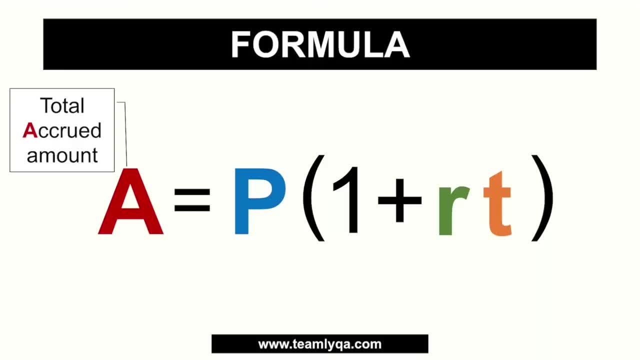 So total amount: okay for A For P, that is your principal amount. If you say principal amount, it means that this is your capital. This is what you invested in the account. Okay now, if this is a loan, that's what you borrowed. For R, that's your rate of interest, And when we 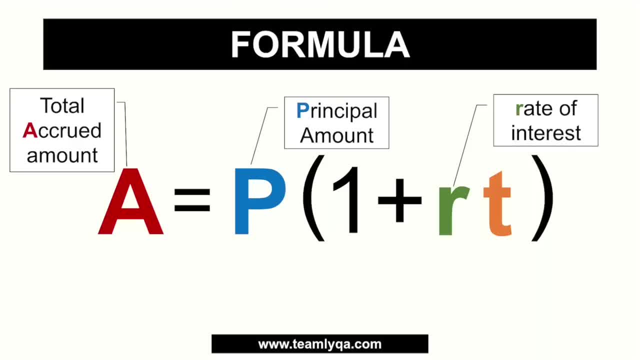 talk about rate of interest. it's in the percentage. We also convert it to decimal. Okay for T. that's the time period. So, for example, two years. you put two there. For three years, three. This is what the formula looks like. 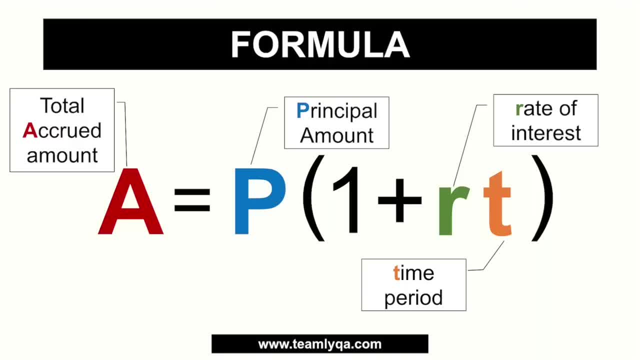 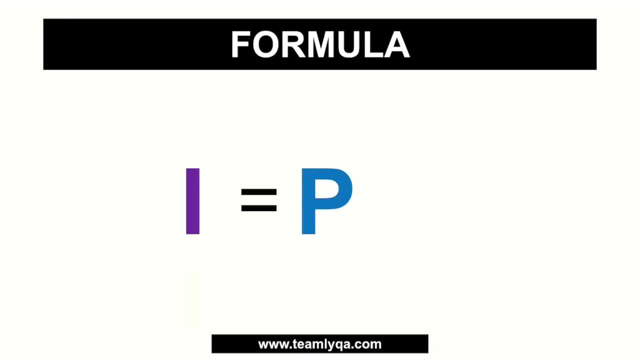 Now there is a simplified version of formula, especially if you're just looking for the interest. If you're just looking for interest or I, what you could use would be the PRT. What the PRT means is that if I is interest, 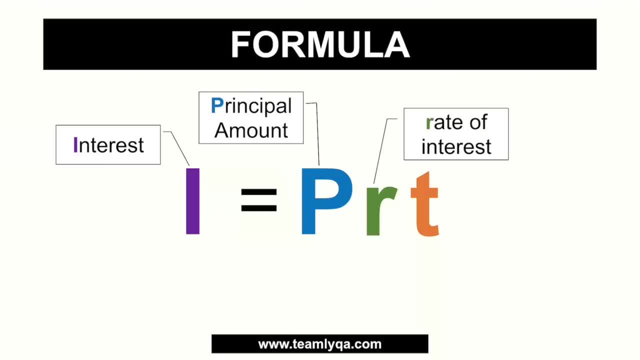 yung P ay yung principal amount, or puhunan Yung R is the rate of interest, Again the percentage, And T yung time period. Now, bakit ganito? Ang idea here is, if you're looking for the total amount, kung total accrued amount, naman lang hinahanap mo ang gagawin mo na lang. 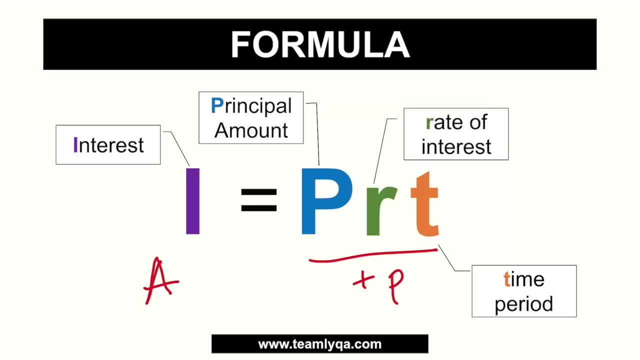 yung PRT, dadagdagan mo na lang ng P Okay. pero kung interest lang hinahanap mo, you use this formula Again: kung accrued amount, same thing, lalagyan mo lang ng isa pang P Okay. 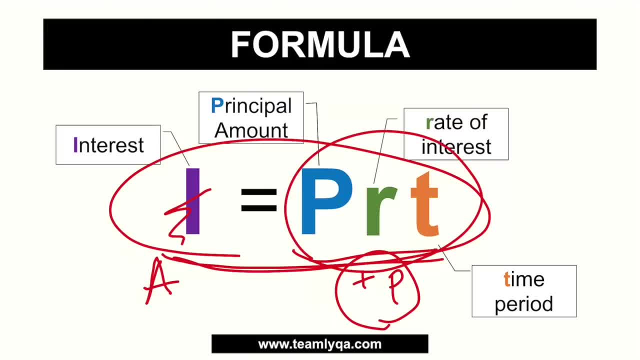 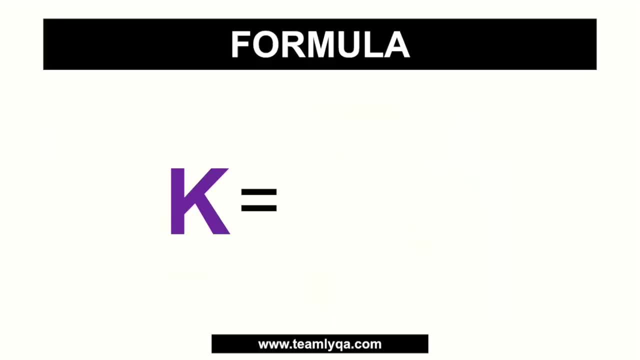 kasi that would be yung pinuhunan, plus itong interest na kinita niya. Now I have another, even more simplified na version nito, which is yung Tagalog. Yung K is equal to PPP. Kaya siya PPP, para madaling tandaan. 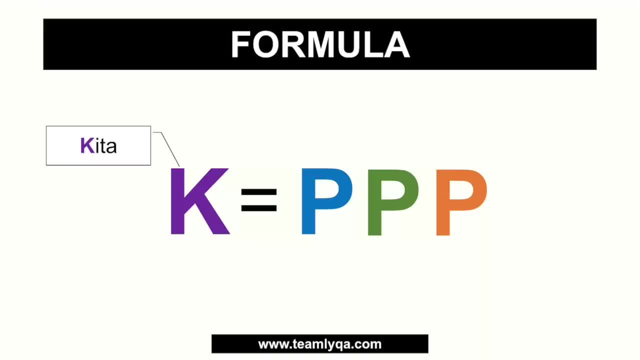 K means kita. So yung kinita mo or yung interest na makukuha mo sa isang account is equal to the puhunan yung pinasok mo na pera times the percentage ng interest rate and then yung panahon. 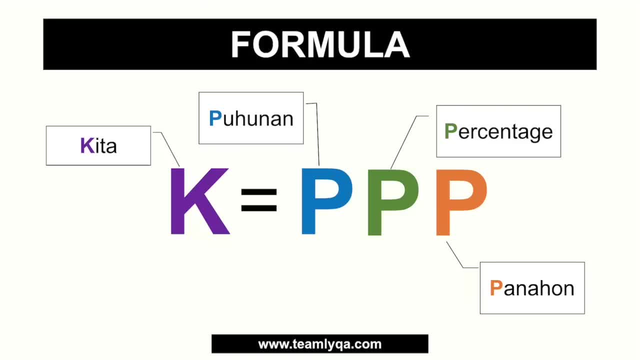 which is yung kung gaano katagal mo siya nilagay doon sa account na yon. So again, KPPP. Now it's almost the same lang din as yung PRT kanina. Yung interest is equal to PRT Iniba ko lang yung. 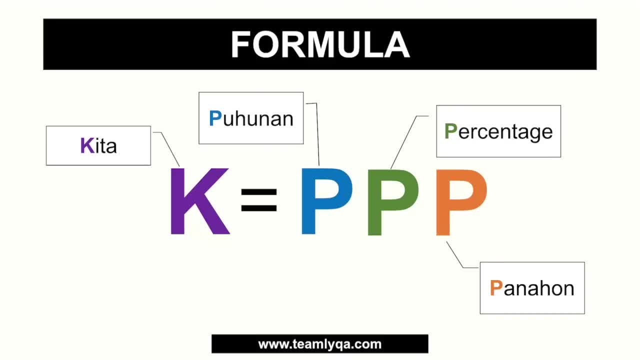 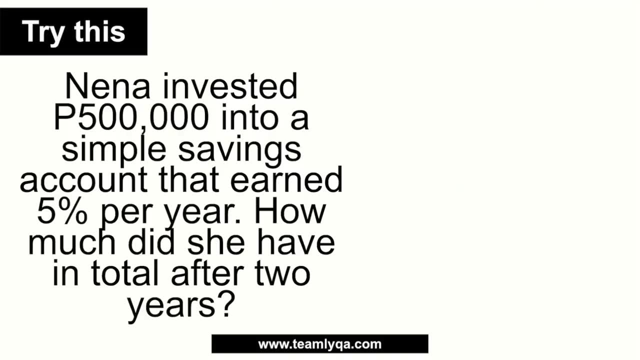 terminology para lang mas madaling tandaan, kasi lahat sila P. Okay, now paano natin ito gagamitin, If you have a question like this? nena invested 500,000 into a simple savings account that earned. 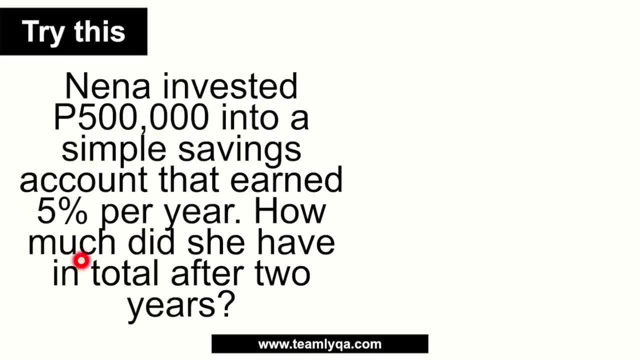 five percent per year, How much did she have in total after two years? Now, if you're going to use yung traditional formula, which is like this: since ang hinahanap naman is total, ibig sabihin, kung total ang hinahanap same yan as yung accrued, Ang una mo kasing. 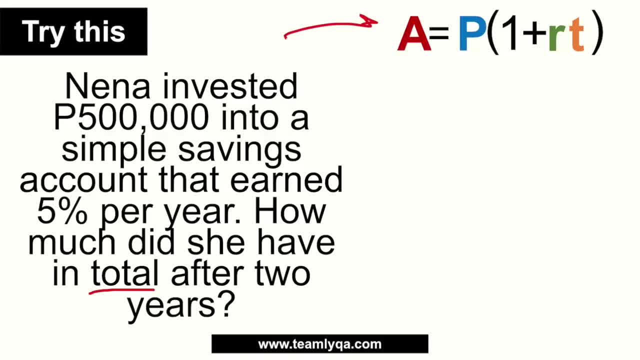 kailangan i-determine ay kung ano ba yung hinahanap. Okay, Kung ano yung hinahanap sa tanong para madaman mo kung anong tamang ipa-plug in mo doon sa formula ng section After you look at kung ano yung. 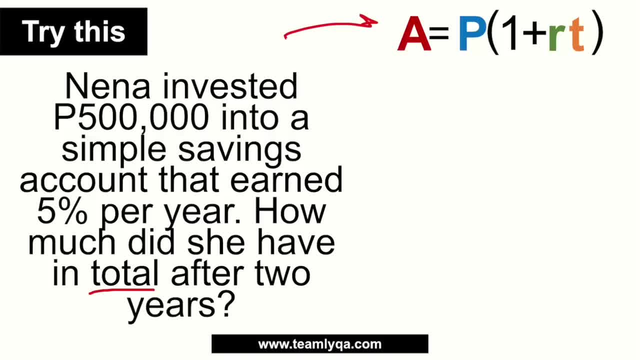 hinahanap, you can start looking at kung ano yung mga binigay Okay. So dahil ang hinahanap natin ay total a, yung hinahanap natin that becomes our x is equal to. And then yung P, ang P natin is the principal. 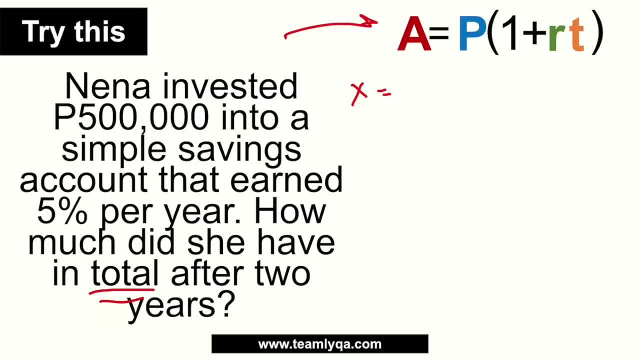 or puhunan. Ang pinasok niya na pera sa kanyang account is 500,000 pesos. So ibig sabihin yung P is going to be five hundred thousand. Okay, and then sabi dito: one plus yung R, naman natin yun yung. 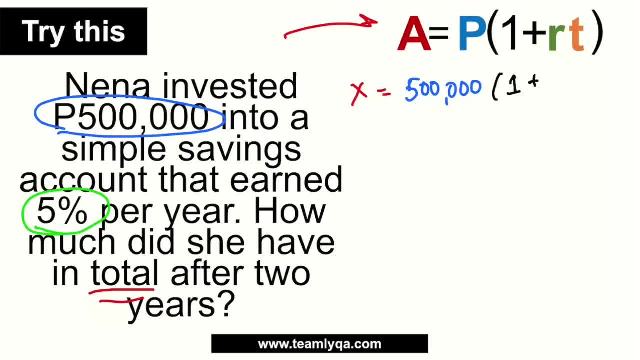 interest rate. Ang interest rate is five percent per year, So ibig sabihin, yung interest rate is five percent per year. So ibig sabihin, yung interest rate is five percent per year. So ibig sabihin: 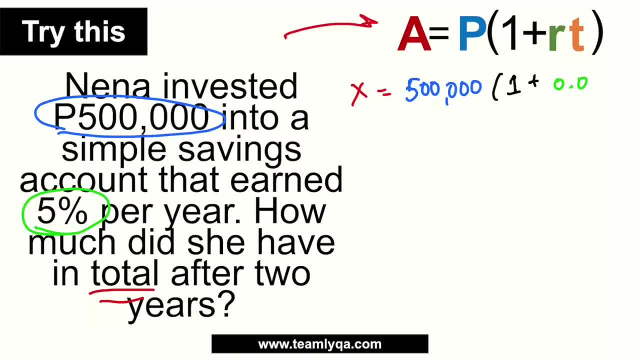 ito: lalagay natin dito 0.05, kasi yan yung 5%. now, if you don't know how to convert percentage into decimal ililink ko na lang din dito yung conversion series natin. ang gagawin mo lang kasi dyan you're. 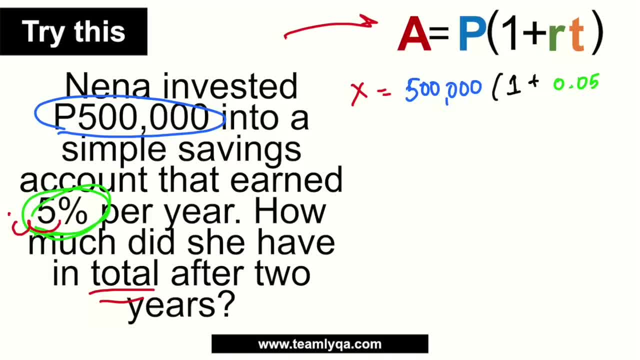 going to basically move the decimal place twice, so magiging 0.05. sya kaya yun ang nalagay natin doon. now yung time naman: ang time is two years, so ibig sabihin i-multiply natin to sa two and then. 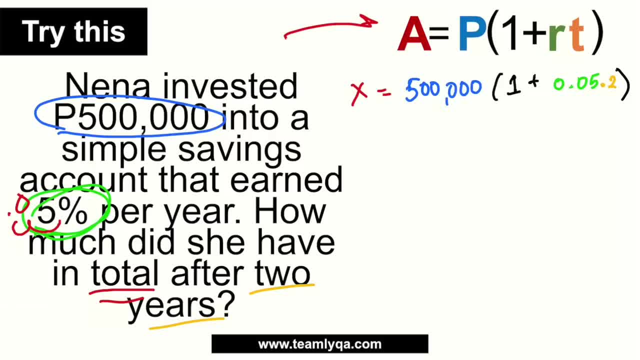 yan yung ating magiging formula. tas isosolve lang natin yan. so kung isosolve natin yan again, we'll just solve down this time. so x is equal to 500,000, tapos 1 plus. now nauuna kasi ang. 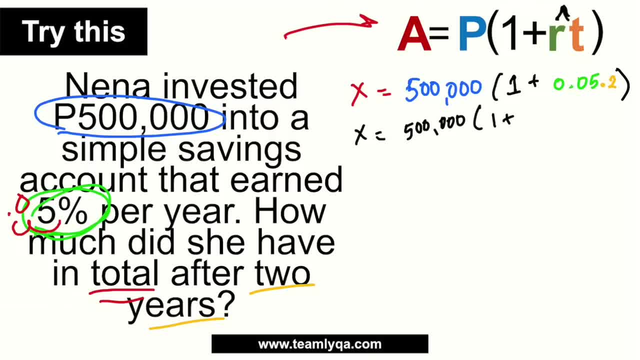 multiplication diba pemdas. multiplication muna bago addition. so i-multiply muna natin to 0.05 times 2. that is going to give us 0.1 or 0.10 or 10 percent. so yan na yan kukopihan ulit natin: x is equal to 500,000 times 1.1. okay, bakit 1.1? kasi this is 1 plus 0.1, that is. 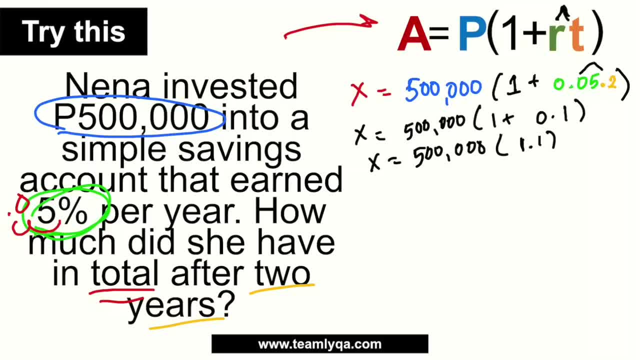 1.1. tapos i-multiply natin yan ngayon. so x is equal to 500,000 times 1.1. now if you solve it long cut, it will look like this: times and then 1.1. so ang gagawin mo, dyan, would be isusulat mo. 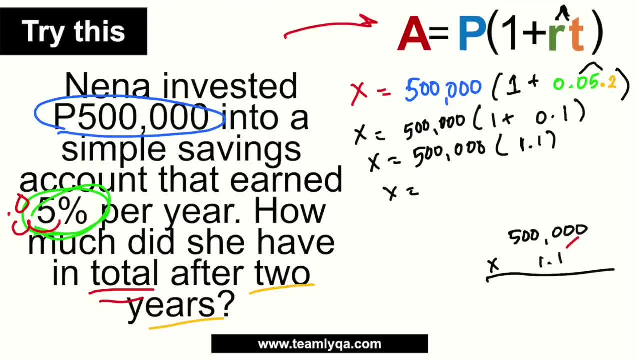 yung 500,000, kasi i-multiply mo siya. eh, so ganun yan diba. okay. so it's going to give you 1, 2, 3, basically sinulat mo lang yung same thing, tapos yung next na level, which is yung dito naman. 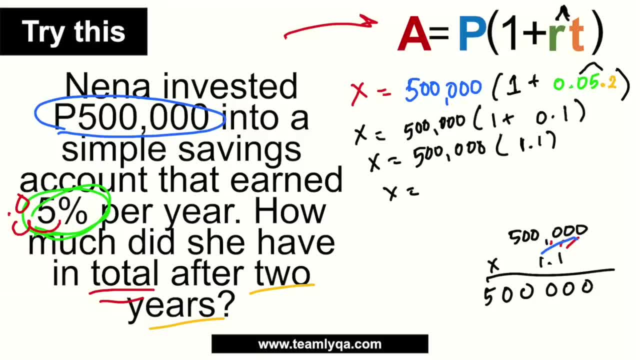 sa 1 na ito. so 0 times 1 same thing lang din. okay, kaya nandito mo na siya ilalagay: 0 0 0, 0 0, 5. i-add mo to lahat, so we have. 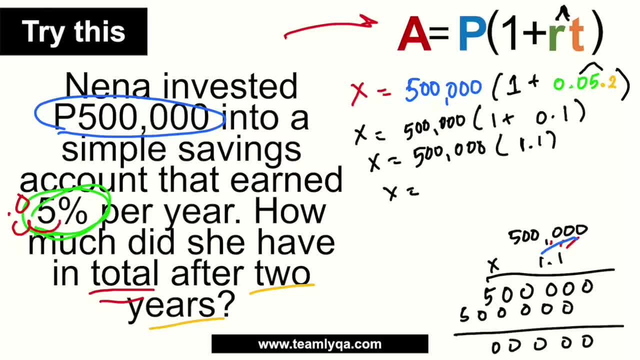 okay, 4, 5, 5, 5, tapos, dahil meron kong isang decimal point, i-move mo yung decimal point kukuha ka ng isa dito, so your answer would be this: 550,000. okay, now, if you know your percentages mas madali, bakit kasi? 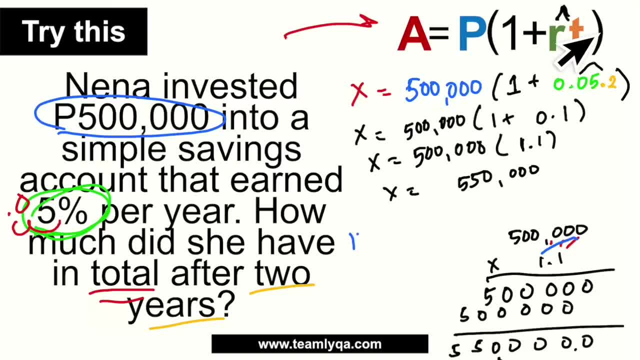 alam natin na ang 10 percent of any number is basically just moving the number, moving the decimal place ng number isang beses pabalik. so kung ang 1.1 is 1, which is yung 500,000, okay, plus 0.1, which is 10 percent, so ang 10 percent ng 500,000. 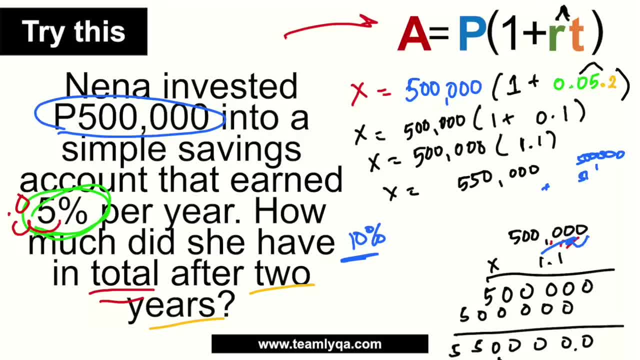 i-move ko lang yung decimal place na isang beses, that is going to give me 50,000. if you notice, mas madali, to just add 500,000 and 50,000, it will still give me 550,000. pareho lang naman din yun. okay, kaya again, kung marunong ako ng estimation when it comes to decimals. 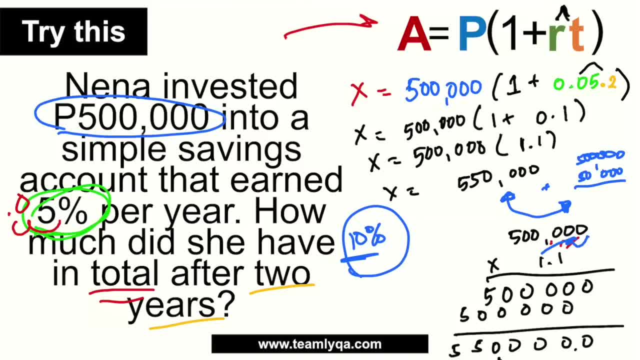 Kaya very important for you to know yung technique when it comes to estimation ng percentages, Lalo na kung may options, mas madali pa yun, Okay, So basically minultiply mo lang sya again sa 1.1.. 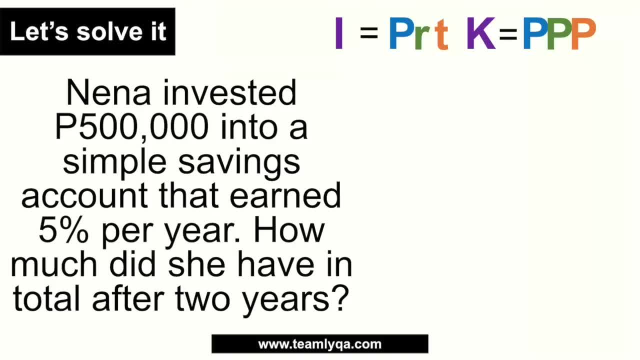 Now let's see if ano yung kailangan natin gawin, kung kunyari ito namang simplified na formula ang gagamitin natin, Kasi parang yung iba, kapag may 1 plus and then RT, yung quantity medyo naguguluhan na sila. 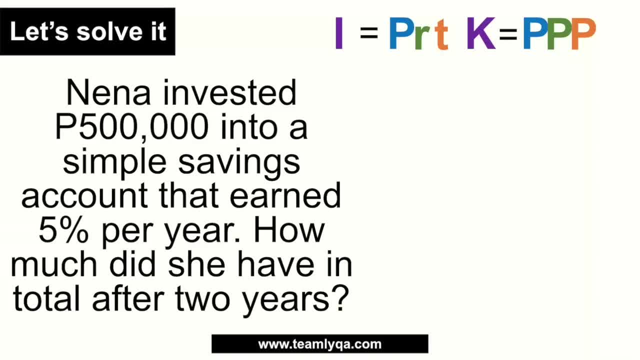 Kung ganitong klaseng formula ang gagamitin natin, anong mangyayari? Now again same thing. ang hinahanap is total. Now, keep in mind: ang total ay ibig sabihin nun yung puhunan or principle, plus yung interest. 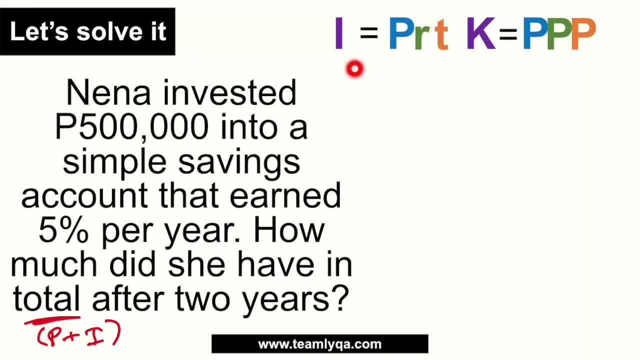 Okay. So ibig sabihin, sa dulo ng lahat ng ito, kapag na-solve na natin yung interest, i-add pa natin yung puhunan. Now, if we solve for yung interest or yung kita, that would be kita. okay, equals yung puhunan, which is the same 500,000,. 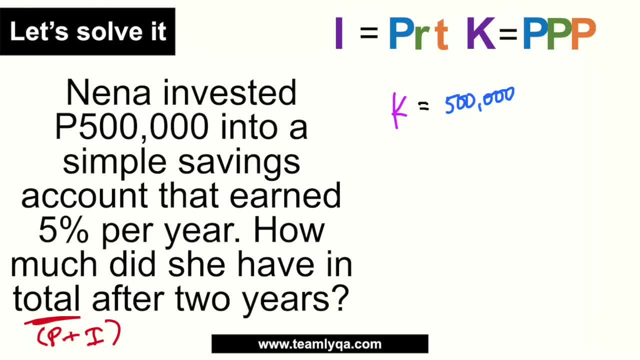 times yung percentage, which is 5%, again that is 0.05.. Times yung time or panahon, which is 2 years, so that is 2.. Again, same thing na gagamitin natin as before. you have your kita is equal to imumultiply lang natin itong dalawang. ito muna mas madali, kasi yun that way. 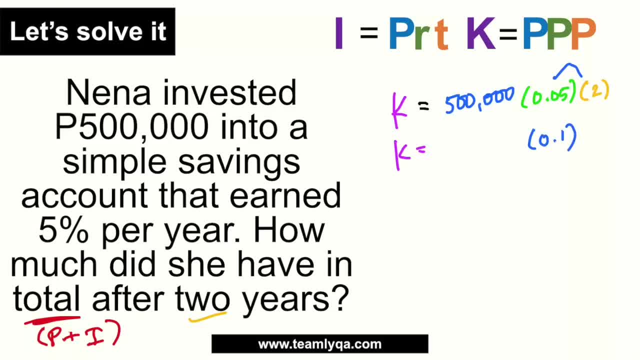 So you have 10% or 0.1 times 500,000.. Now, kung 10% na yan kasi ito, it's the same thing. it's still 5% times 2, parang 5% times 2 is 10%. 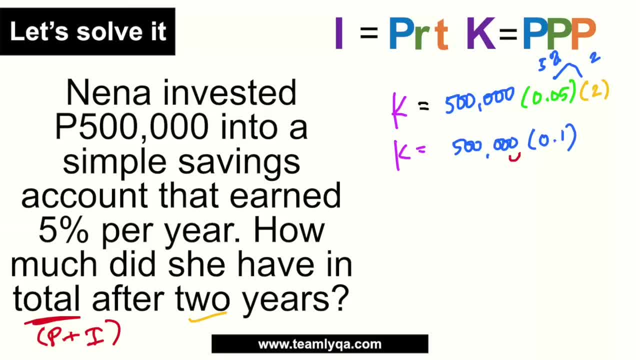 So, again, using yung ating estimation ng decimal, imumove ko lang yung decimal place na isang beses kita natin will be 50,000.. So kung total ang hinahanap, dadagdag lang natin yung ating pinuhunan, which is 500,000,, lalabas pa rin same thing: 550,000.. 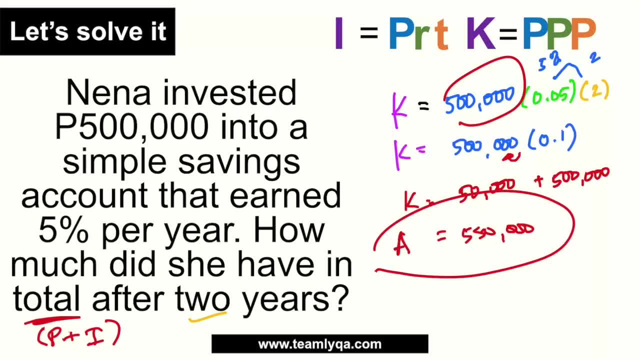 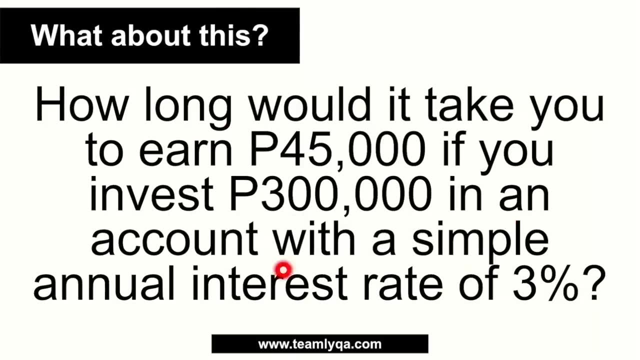 Yun yung total or accrued amount. yun ang magiging sagot. So same thing again, whether dumaan ka dun or dito. Now paano, kung ganito Sabi dito, how long would it take you to earn 45,000 pesos if you invest 300,000 in an account with a simple annual interest rate of 3%? 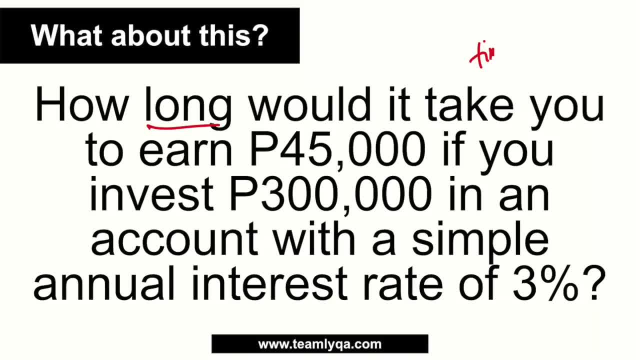 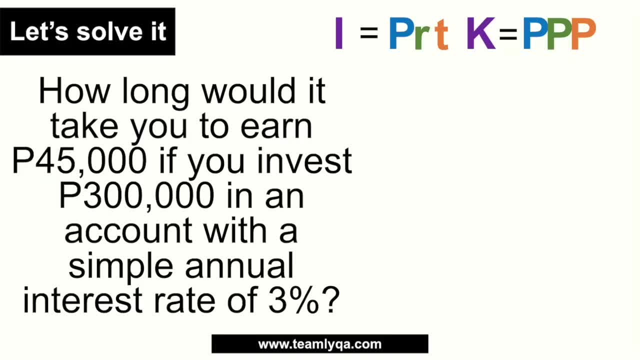 So ang tanong is: how long? Ibig sabihin we're talking about time, Time ang nawawala this time. So ang first question would be: which formula am I going to use Ang sabi dito: how long would it take you to earn? 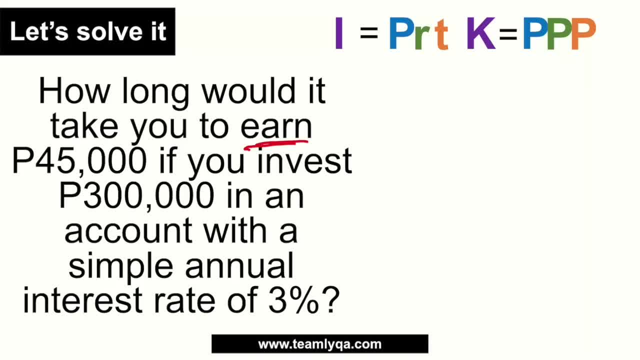 Ibig sabihin ang earn kinita mo siya. So I cannot just use yung formula for accrued Yung total amount, kasi hindi naman interest yung binibigay dun, Binigay na yung halo ng lahat. 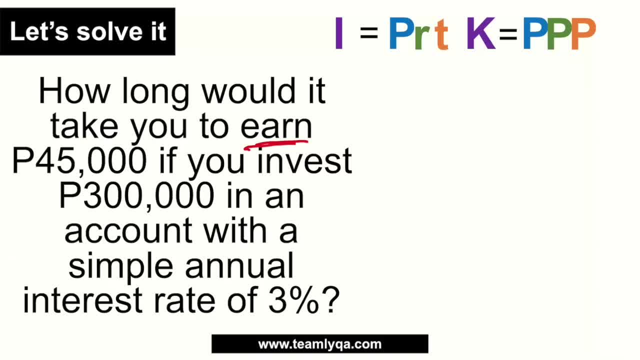 So mas madali sa akin to use yung simplified na formulas natin here. 45,000, yun yung kinita. Okay, so fill in ko lang siya: 45,000 is equal to okay. 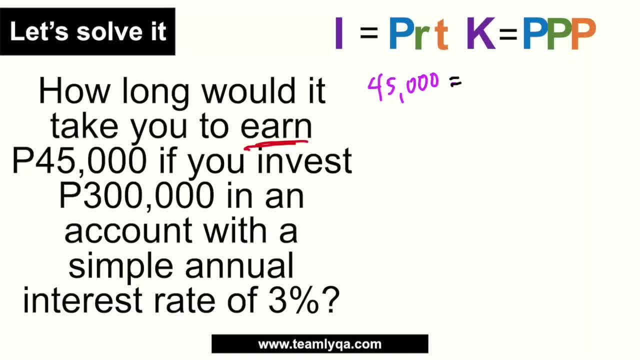 ang ating puhunan ay 300,000.. So yun yung ilalagin natin dito First, 300,000.. Tapos, yung kanyang interest rate ay 3%, 0.03.. 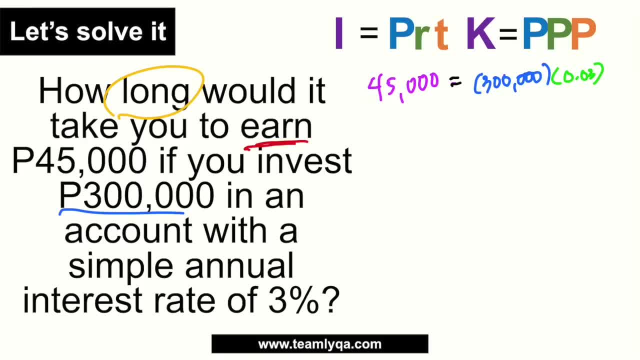 Ang nawawala is how long. So ibig sabihin yun yung magiging x natin this time. So dito na nagiging medyo mas tricky yung things, Kasi nagiging mas complicated yung pagsosolve kapag yung x ay nagpalipat-lipat na ng pwesto. 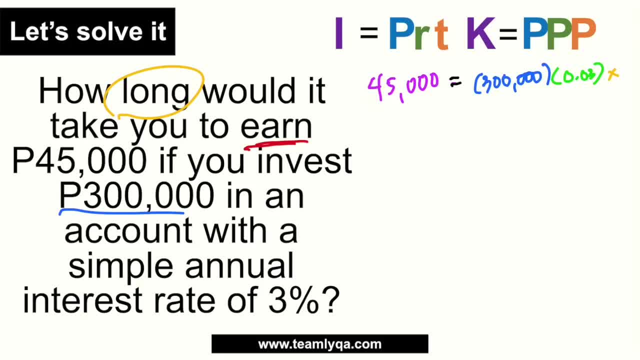 Pero if you're going to use algebra, same thing lang din. Yun pa rin ang gagawin natin. So ibababa lang natin lahat yan, Iko-combine. natin, yung mga kailangan natin, i-combine. 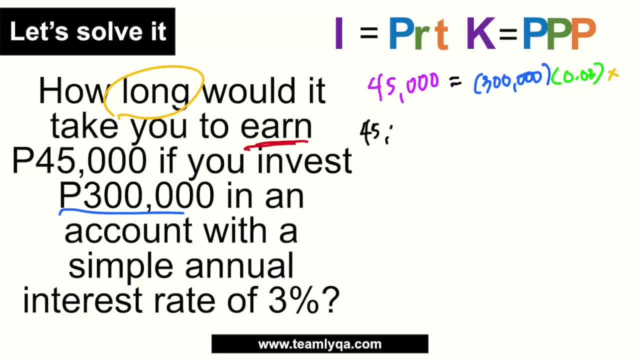 So here You have 45,000 pa rin. So solve na natin: Is equal to Now yung 0.03x. hindi muna natin masosolve yan ngayon, Kasi wala naman tayong pwedeng gawin dyan. 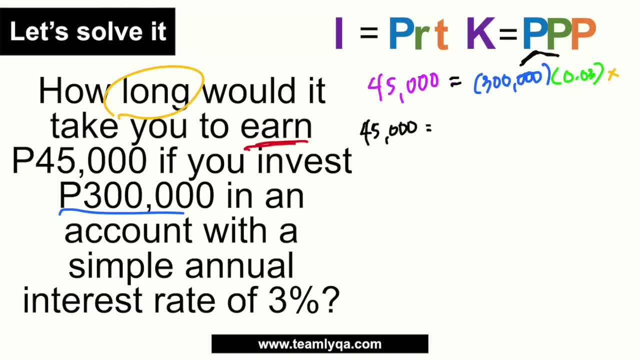 Pagtatabihin lang natin siya Ito, pwede natin siyang isolve. So ano ba ang 3% ng 300,000?? Now again pwede nyo i-multiply yan As in 300,000 times 0.03.. 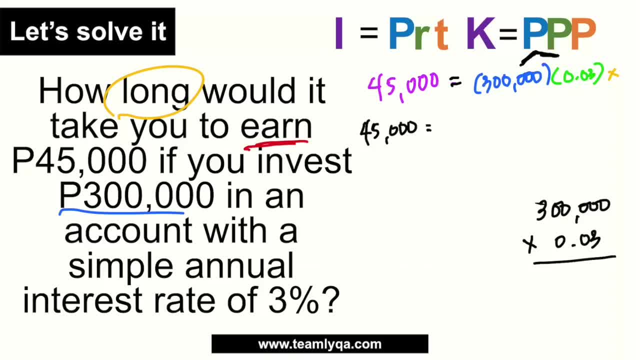 Or kung magaling ka mag-estimate or mag-guestimate, you would know na ang 3% okay. Kung ang 10%. ang 10% is just moving the decimal place one time. ang 1% would be moving the decimal place two times. 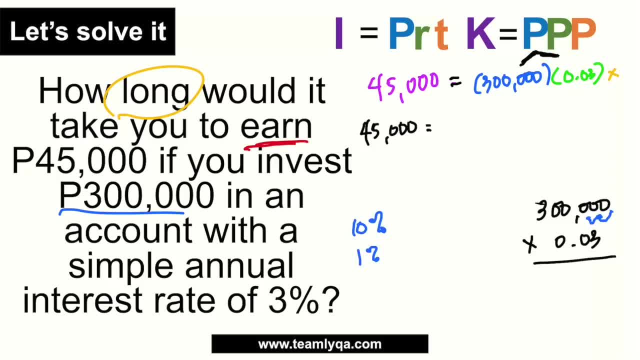 So ibig sabihin ang 1% ng 300,000 is 3,000.. Okay, Bakit Kasi nag-move ako ng decimal place Twice, So ang naiwan is 3,000.. 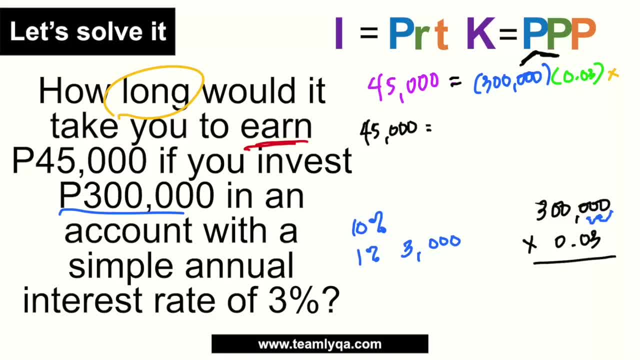 3 and 3,000.. Yan ang 1%. So kung gusto ko hanapin yung 3%, ang kailangan ko lang gawin is to add 3,000, or i-multiply ko na lang siya sa 3.. 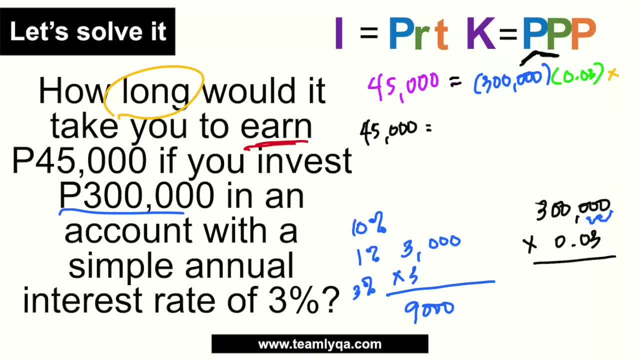 That will give me 9,000.. So ibig sabihin, ang 3% of 300,000 is actually 9,000.. And then i-dikit ko na lang yung x. Now to solve this, I'm going to add 3,000.. 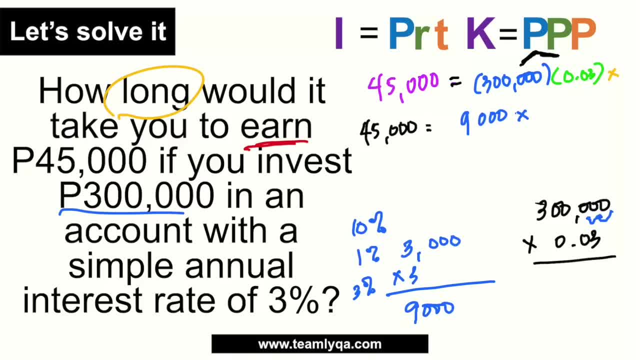 Now to solve this, I'm going to add 3,000.. So ibig sabihin, ang 3% of 300,000 is actually 9,000.. Now for x, para makancel ko yung 9,000 dito sa right side. 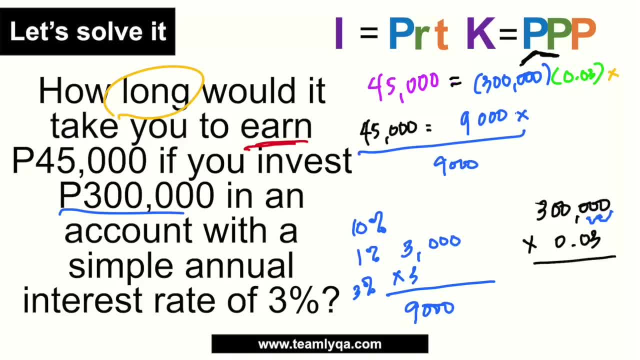 i-divide ko yung both sides by 9,000.. Maka-cancel, ito x is equal to 45,000 divided by 9,000.. At ilan yun, That is basically 5.. So ibig sabihin x is equal to 5.. 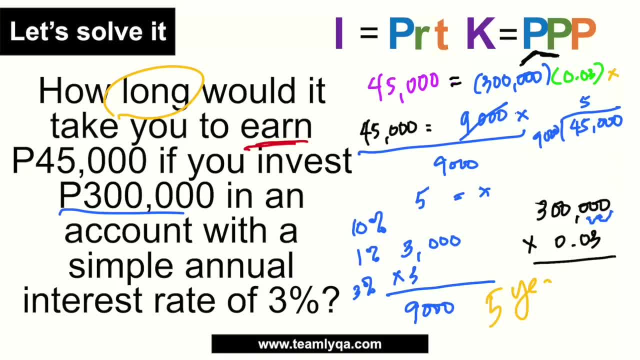 The answer is 5 years. Okay, So yun yung kumbaga hopes. So yun yung kumbaga hopes. So yung, yung kumbaga hopes. So yun yung kumbaga hopes. 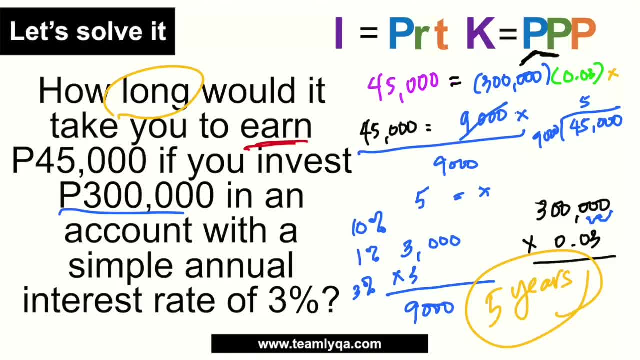 So yun yung kumbaga hopes. So yun yung kumbaga hopes. Now again, whether you multiplied it like this and divided it like this, or kung gumamit ka ng estimation tapos tsaka ka nag-cancellation naman when it comes to your fractions, 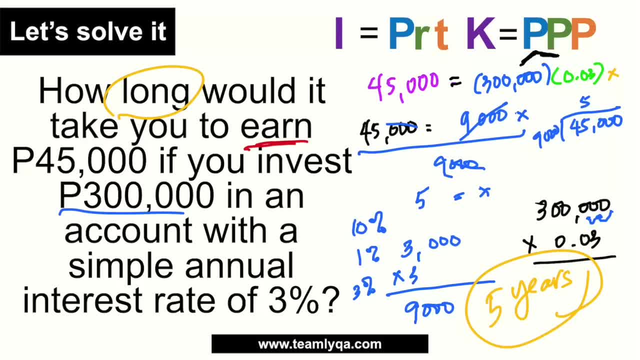 kasi pwede mo i-cancel ito and then divide this na lang: 45 divided by 9 is 5, that would be the same answer: 5 years pa rin. Kaya lang. mas maganda kung equipped ka with yung mga skills nito. estimation. 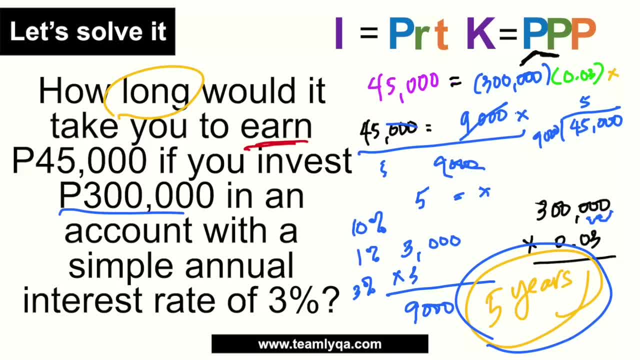 kung marunong ka mag-fractions by cancellation, ililingko na lang din dito sa taas para makuha ninyo yung technique na yun, Kasi that will help you a lot when it comes to solving more complicated word problems. 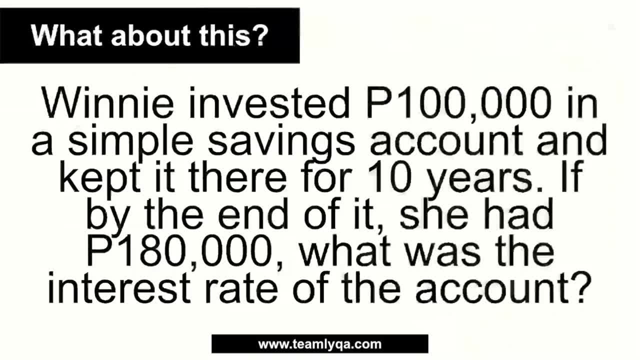 Now paano naman, kung ganito? yung tanong: Sabi, when he invested 100,000 in a simple savings account and kept it there for 10 years, if by the end of it she had 180,000, what was the interest rate of the account? 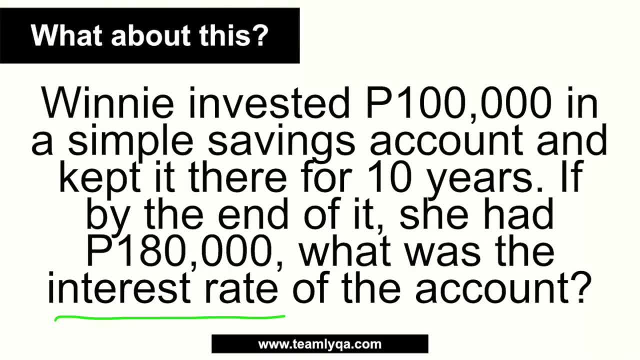 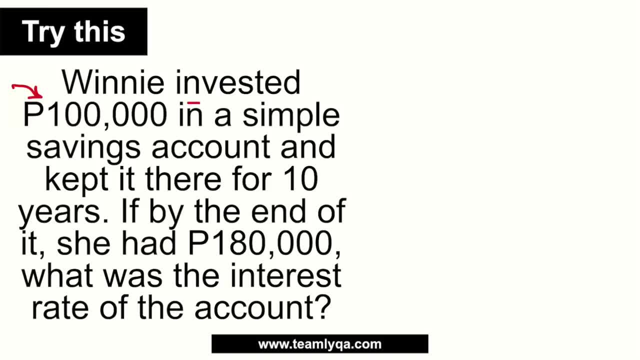 So this time ang hinahanap is the interest rate. What do we do Now, dahil ang binigay sa atin 100,000, yung kanyang ininvest 180,000, ang pera niya at the end. so ito na ang total. 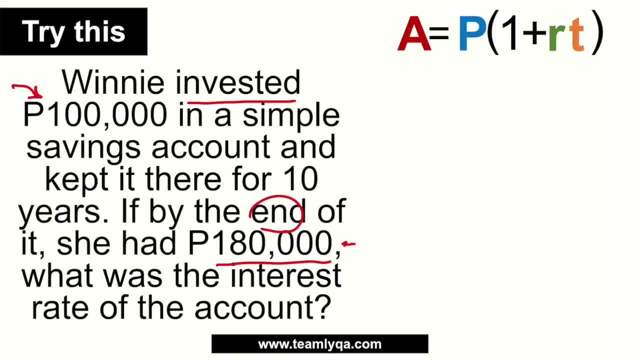 pwede natin gamitin yung formula na ito, which is yung for the accrued amount. So anong gagawin natin dito? We're going to solve it down. ilalagay lang natin yung information na binigay. 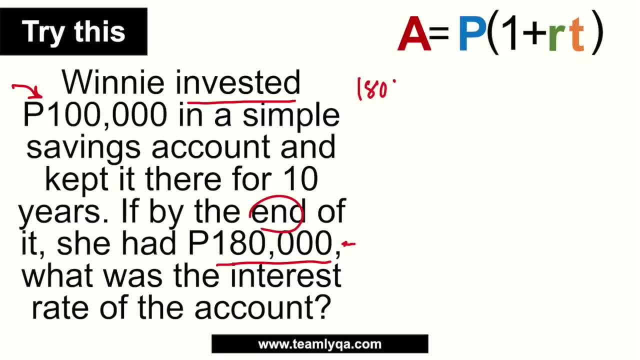 So ang accrued amount natin is 180,000.. Okay, Tapos equal siya dun sa principal. Ang principal natin is 100,000.. Yun yung ininvest, Tapos meron kang 1 plus yung R or rate, yun ang nawawala. 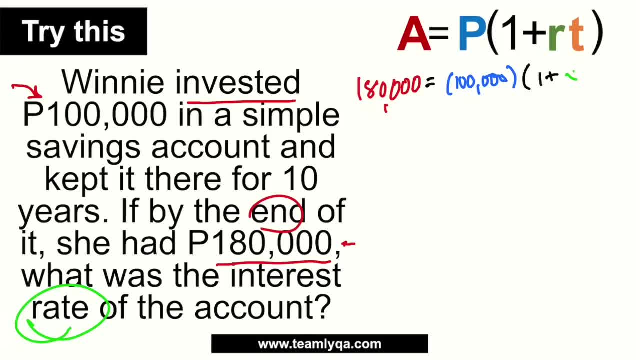 Hinahanap what was the interest rate. So ibig sabihin siya ang magiging X natin this time, And then yung time period natin ay 10 years, So ibig sabihin this will be 10.. 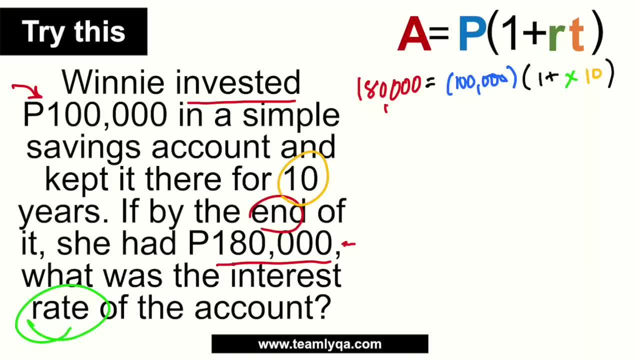 Okay, Tapos magsosolve lang tayo for X. So again it gets a little bit more complicated, dahil nasa kabilang side na yung X, Pero isosolve pa rin natin As we would yung any algebra question. 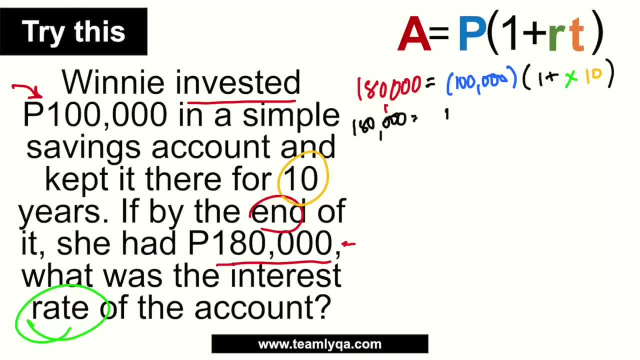 So 180,000 is equal to 100,000.. Tapos isort out muna natin yung nasa loob. So this is 1 plus 10X. Now when we're multiplying numbers, pagdating sa ganito, dalawa yung terms na nasa loob. 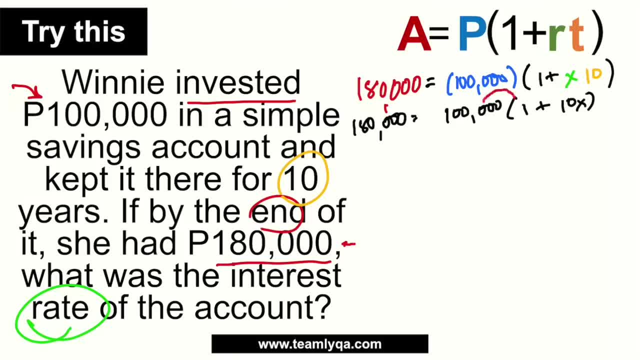 ididistribute natin yung 100,000.. So yung 100,000, imumultiply ko sa 1.. Tapos imumultiply ko rin siya sa 10X. So ibig sabihin nun: 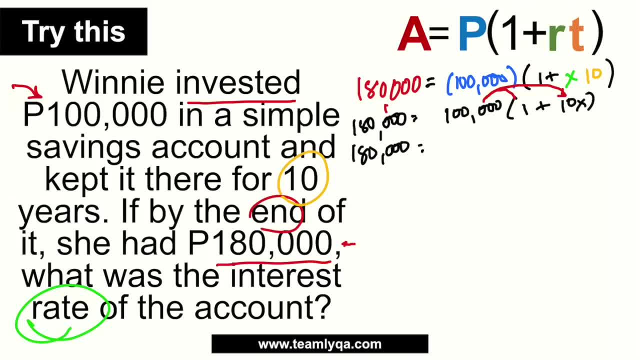 X level natin would be: 180,000 is equal to 100,000 times 1.. That's the same, So 100,000 plus, and then you have 100,000 times 10X, So that would be 100,000. 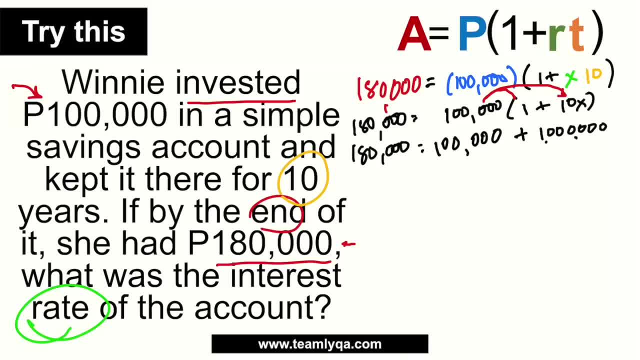 Dadagdagan ko pa ng isa pang zero, So magiging 1,000,000 na siya X. Okay Now, in order for me to leave yung X sa isang side, which is our goal when it comes to algebra, 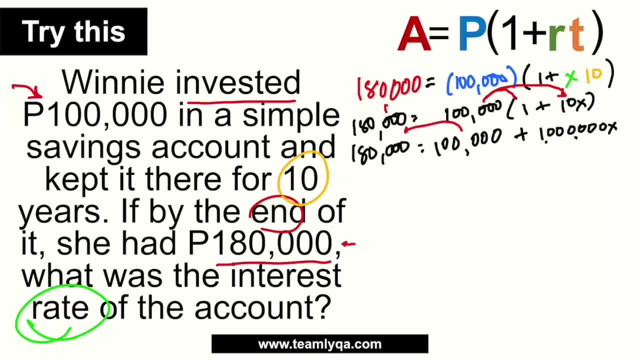 ang gagawin ko yung 100,000.. Na ito ililipat ko sa kabilang side. So ibig sabihin ang mangyayari dito magiging 180,000 minus 100,000 equals 1,000,000X. 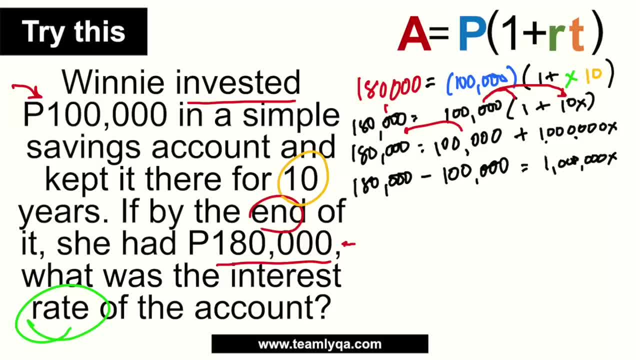 So ang lalaking number yung pinag-uusapan natin dito, Kaya yung iba natatakot talaga sa investment problems. So 180,000 minus 100,000, that is 80,000 is equal to 1,000,000X. 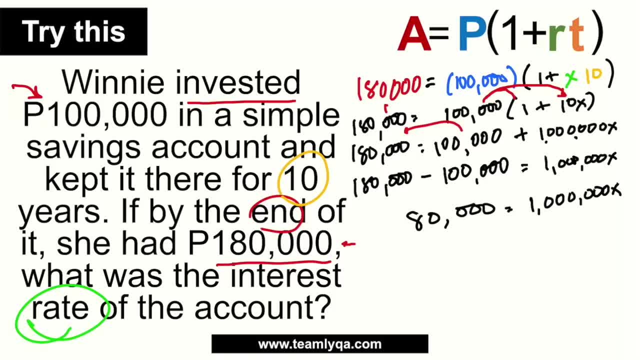 Now to solve for X. what we need to do now is to divide both sides by 1,000,000.. Para makancel ito maiwan yung X sa isang side. So ang dilema na natin magiging 80,000 divided by 1,000,000.. 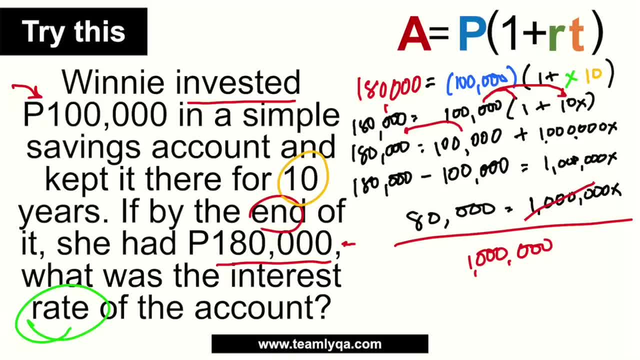 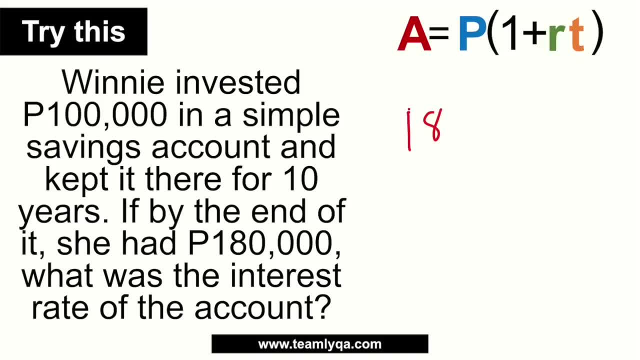 Now the first thing that we're going to do is to cancel na yung mga zero: Apat dyan, Apat dyan. So you are now left with 8 divided by 1.. So ito, isosolve na lang natin. 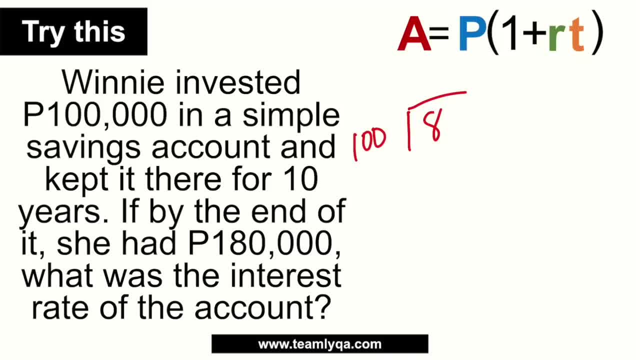 So ang gagawin natin, dyan, dahil we're dealing with decimals- and this is the more confusing part- Lalo na kung wala kang calculator. Kung may calculator ka madali, eh, Pero kung wala kang calculator, isosolve mo ito like this: 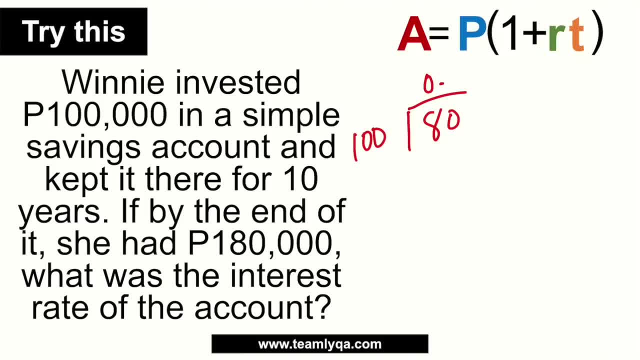 Ang mangyayari, dyan, would be lalagyan mo na mga decimals. So unang decimal will give you that, Another decimal will give you this, And now you can divide it. So 800 divided by 100 is 8.. 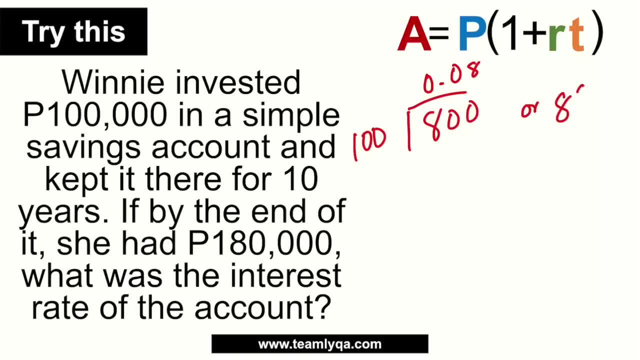 Okay, So the answer is 0.08 or 8%, Or, kung alam mo yung technique natin when it comes to dividing numbers by 10, di ba ang sabi natin kapag nagmumultiply tayo ng number. 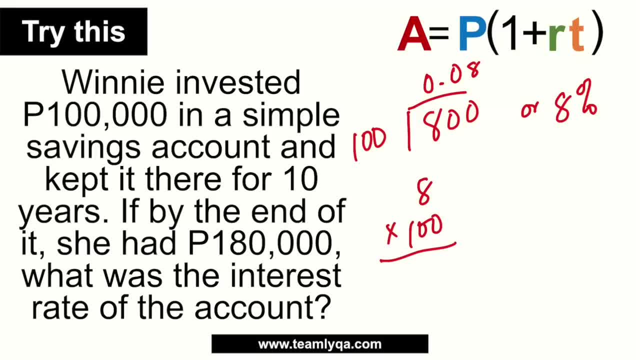 So for example, 8 times 100.. Pag nagmumultiply tayo ang ginagawa natin, dinadagdag lang natin yung zero dito. So dalawang zero dinagdag natin dito. 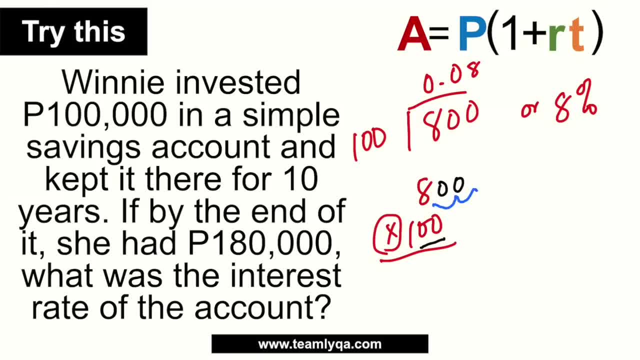 It's basically us moving the decimal place twice. Okay, Dalawang zero dalawang beses. mo rin siya imumultiply, The answer is 800.. Now kapag nagdidivide ka naman ng numbers by multiples of 10.. 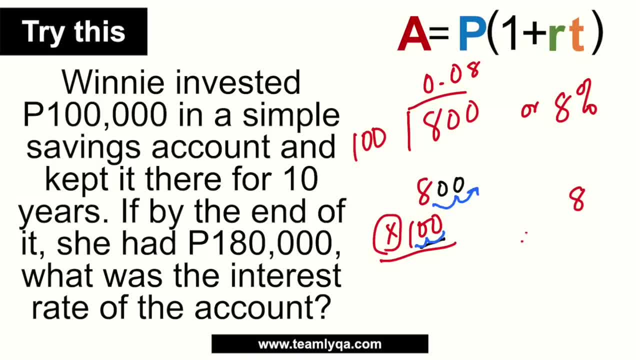 So, for example, in this case, di ba you have 8.. Tapos divided by 100.. Ang pwede mo naman gawin is kabaliktaran nung ginamama pag nagmultiply ka, Kung nagmultiply ka at nagmove ka ng para right. 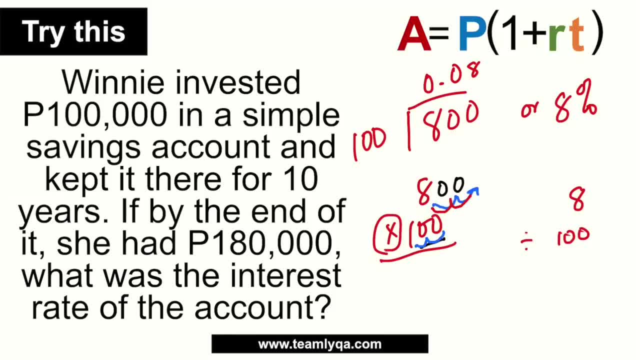 ang gagawin mo naman. kapag ikaw ay nagdidivide, you can move it to the left Sa kung ilan yung zero, So 1, 2.. So 0.08. again Same thing naman. 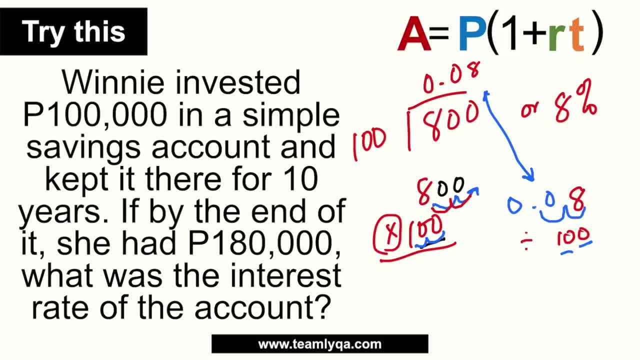 Ang kinalabasan kaysa doon sa naglongkat akong division. the answer will still be 8%. So the answer here is 8%. Now again, that is what you're going to have to do kung naglongkat ka. 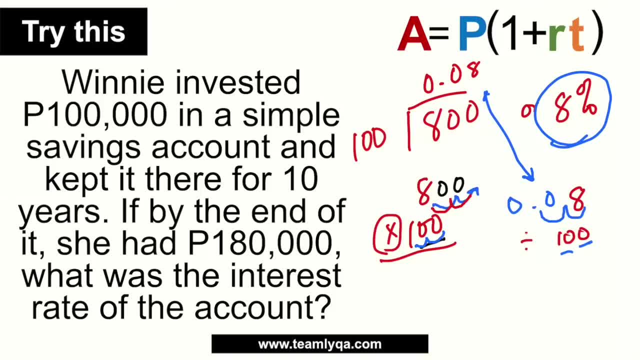 kung hindi ka masyadong magaling mag-estimate at kung walang options Now using yung simplified formula, kung ayaw mo na masyadong malalaking numbers, anong pwede natin gawin? 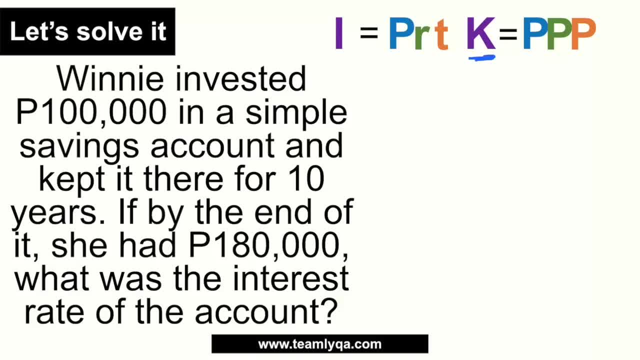 Okay, Ang una mong hahanapin would be: magkano ba talaga yung kinita? Kita lang Now ang sabi sa problem: invest ako ng 100,000, ang ending naging 180,000.. 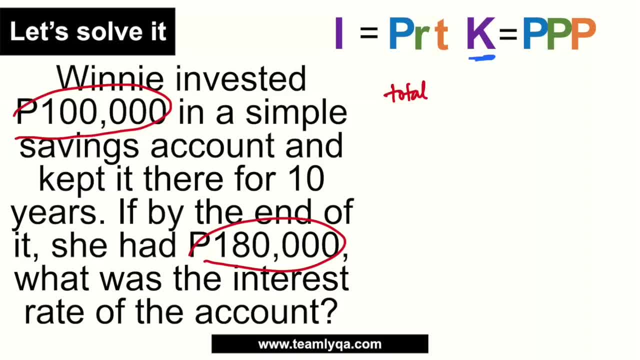 So kung ang total is 180,000, okay, at yan ay equal sa puhunan plus yung kinita. kung ang puhunan ko ay 100,000, okay, magkano ngayon ang kinita ko? 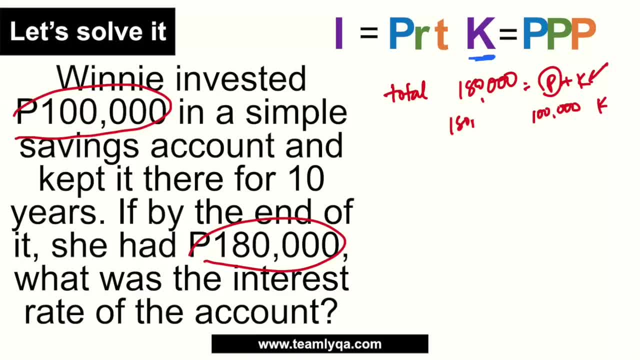 So ang kita ko ngayon is equal to 180,000 minus 100,000 or 80,000.. Ang kinita ko ay ay 80,000 lamang. So ibig sabihin nun, now that I know kung ako, magkano yung kita? 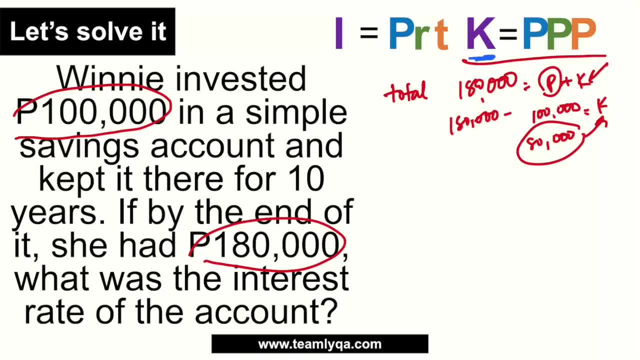 pwede ko na subukan yung mas madali or simplified na formula ang gamitin, So I can write it down: Ang kita ko is 80,000.. Okay, Equal siya sa puhunan, which is yung 100,000 initial na investment. 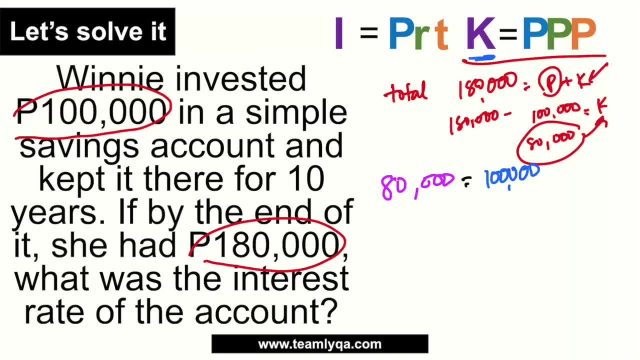 times the percentage which is hindi natin alam, So that would be your X. And then yung panahon natin, ang panahon natin ngayon may 10 years, So that would be 10.. 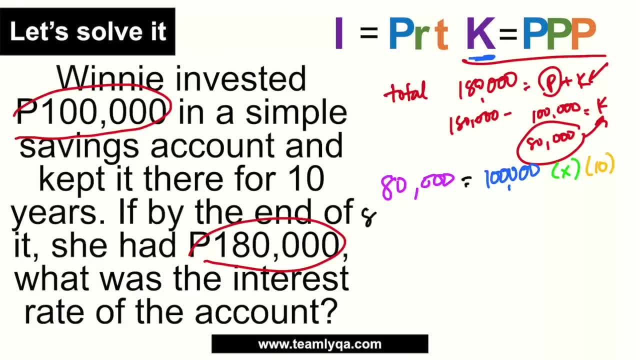 So now you have solving it down: 80,000 is equal to 100,000 times X, times 10.. So again, babalik tayo dun sa 1,000,000 na siya. Okay, 1,000,000 X. 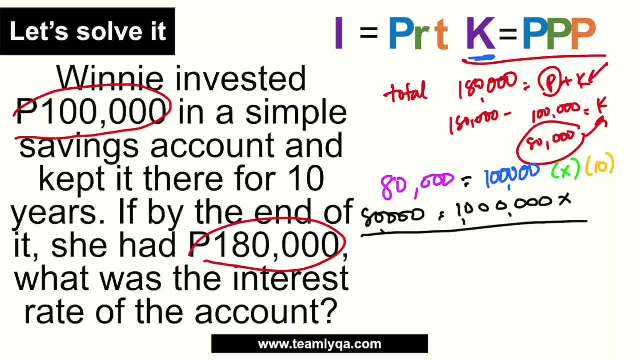 Shortcut lang siya ng konti, kasi didiret siya na ako ngayon sa pagdidivide ng 80,000 sa 1,000,000.. Instead of going through the hoops na may ima-minus pa ako. 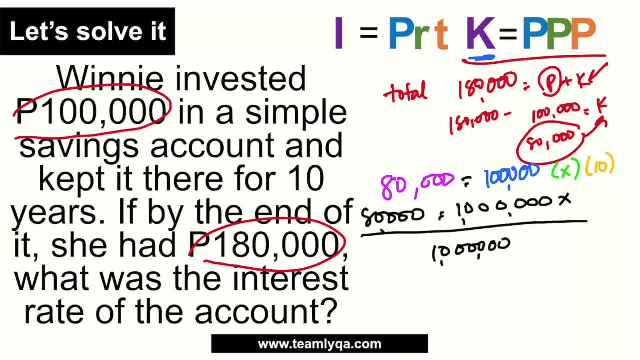 may itatranspose pa ako. Again, i-divide ko lang yan, i-cancel ko to. So X is equal to 80,000 divided by 1,000,000.. Again, same thing. cancel to cancel. yung apat na zero dyan. 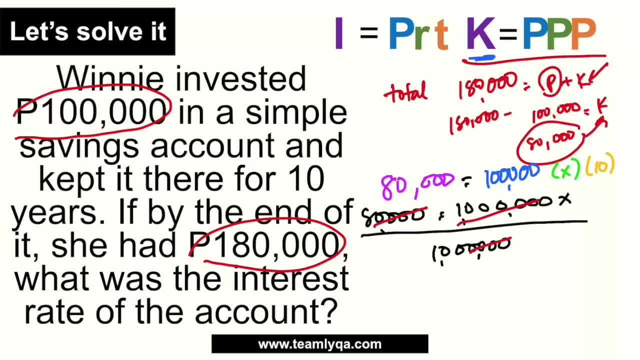 Kung nako-confuse kayo dyan, inilink ko dito sa taas yung multiplying fractions by cancellation. Panoorin nyo na lang yun. So now you have again same thing: 8 divided by 100..